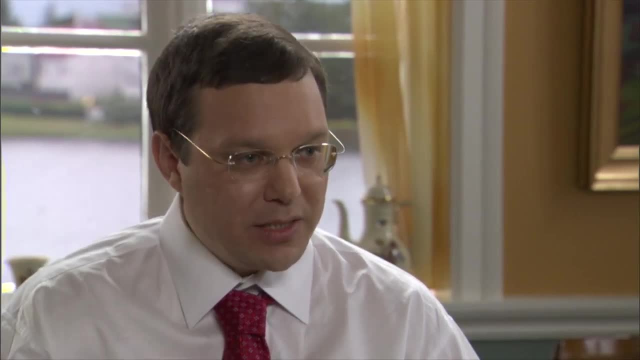 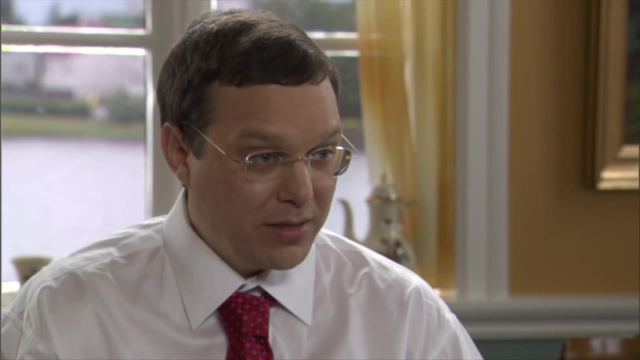 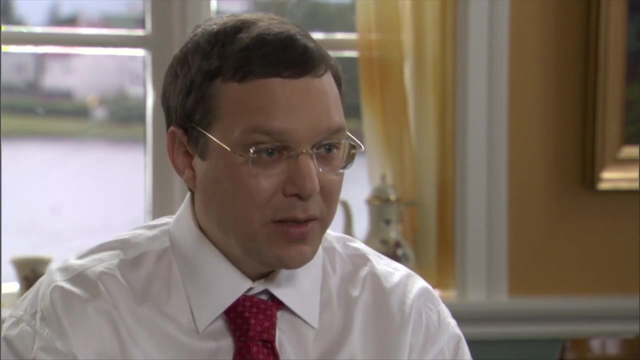 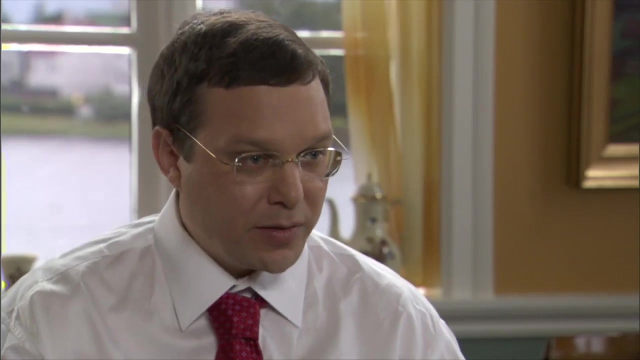 The way to do that is by looking for a transition, atomic transition of hydrogen that corresponds to a wavelength of 21 centimeters. in the radio, And because of the expansion of the universe since that time that we are trying to observe, this wavelength is being stretched to meter size, comparable to the height of a person. 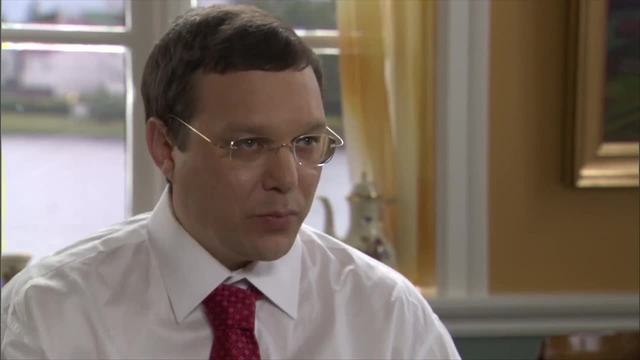 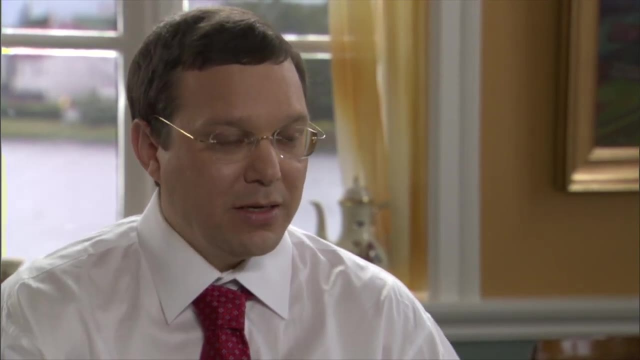 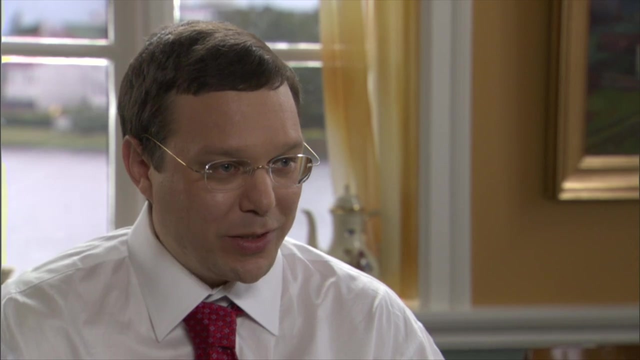 Another way to put it is that the frequencies that one is looking for are about a few hundred million hertz, 100 megahertz. You find those frequencies on your radio dial. These are the kind of frequencies we are using for radio and TV communication. 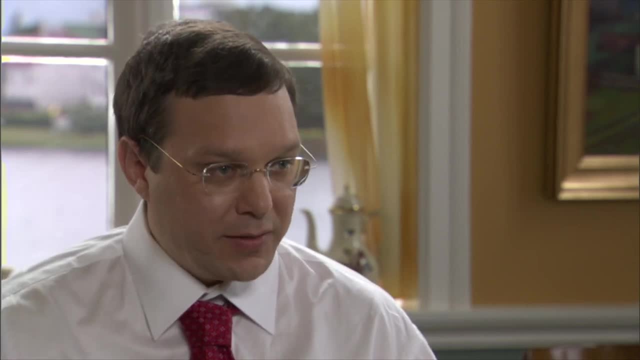 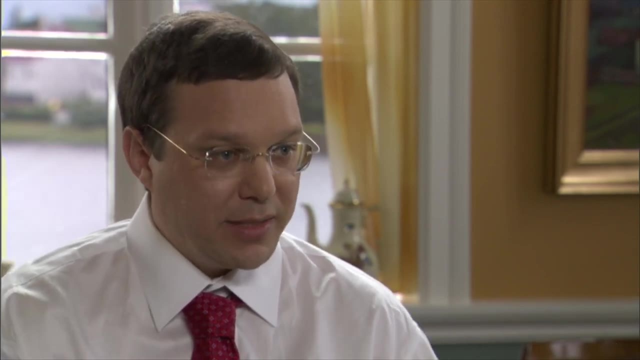 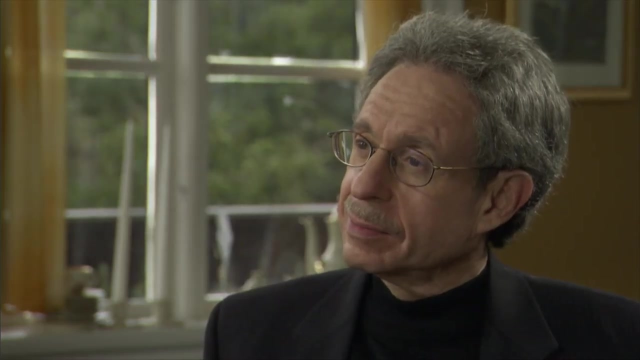 And so the goal is to develop very large arrays of radio antennas, each of which that contains about 10,000 such antennas that look just like the antennas you can buy for a television reception, and put a large number of them across a field that is a kilometer size. 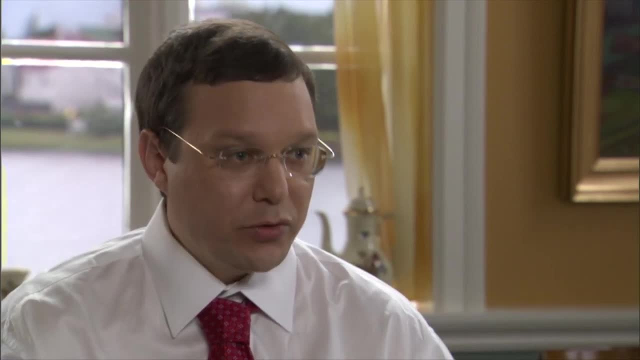 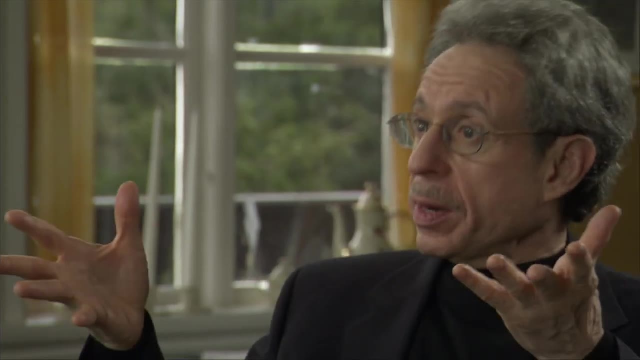 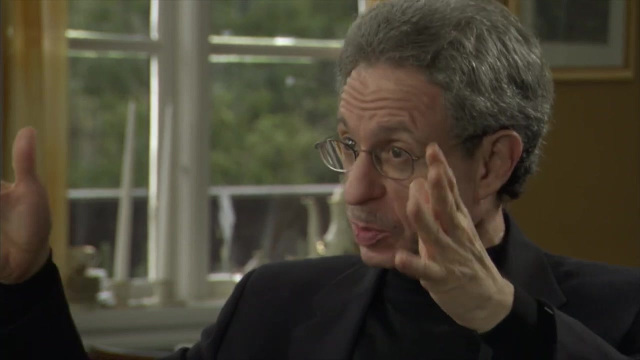 And you link all these antennas And try to image the 21 centimeter transition of cosmic hydrogen from very early times. So simulate what it might look like if we did those imaging for that time. We're imaging the hydrogen that occurred Now. what years approximately are we dealing with that you're seeking the image from? 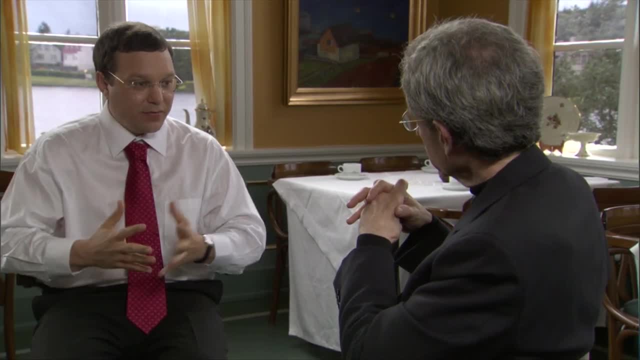 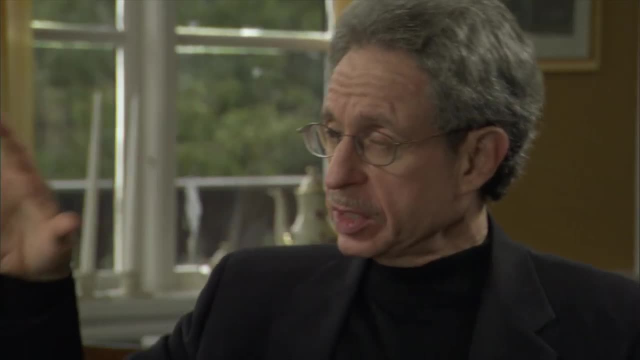 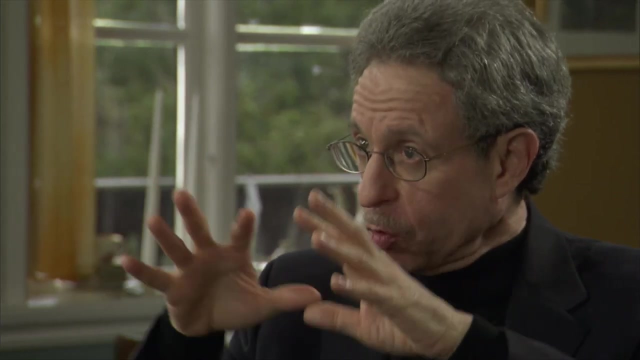 We are talking about the time that preceded the first billion years, So we're talking about hundreds of millions of years after the Big Bang, And we're imaging the The distribution of hydrogen at that time, because that would give us the first indication of how structures were being formed. 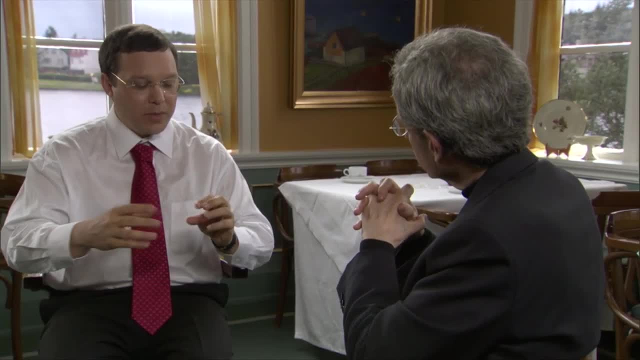 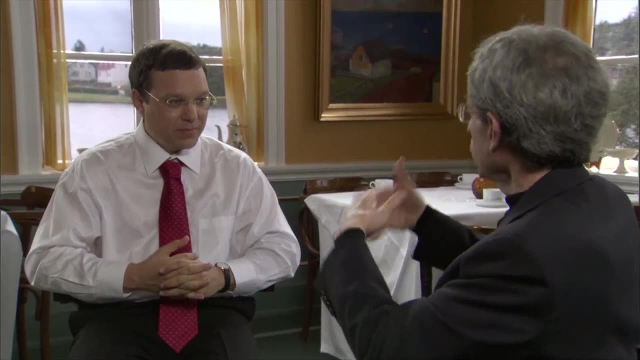 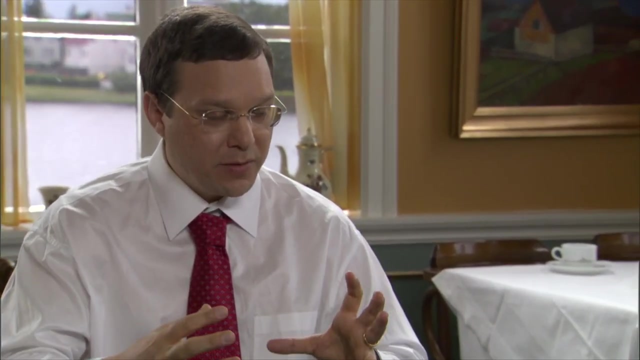 Exactly Now. the hydrogen early on was not uniform because of the inhomogeneities that resulted from inflation, From the quantum fluctuations within inflation. That's correct, Right. But then when the first galaxies formed in the universe, they produced radiation that broke the hydrogen atoms in the vicinity of these galaxies. 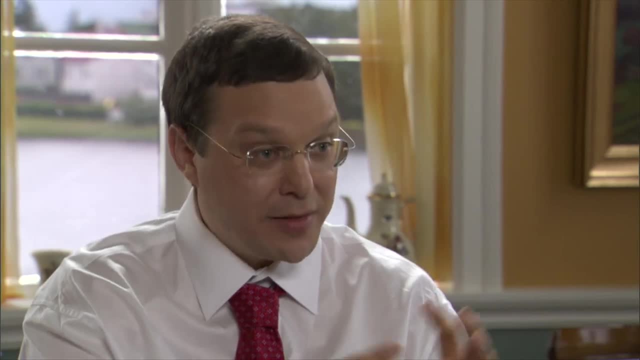 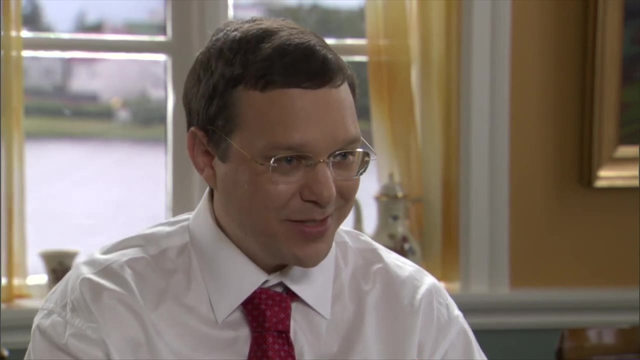 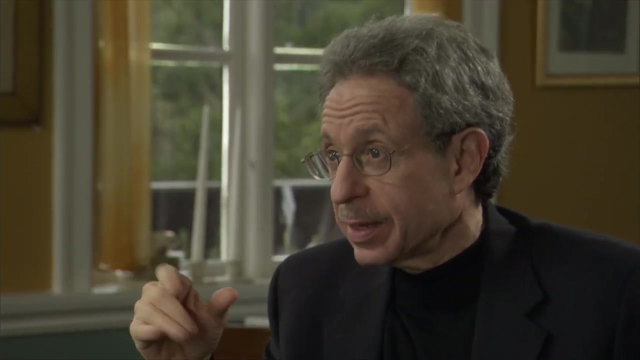 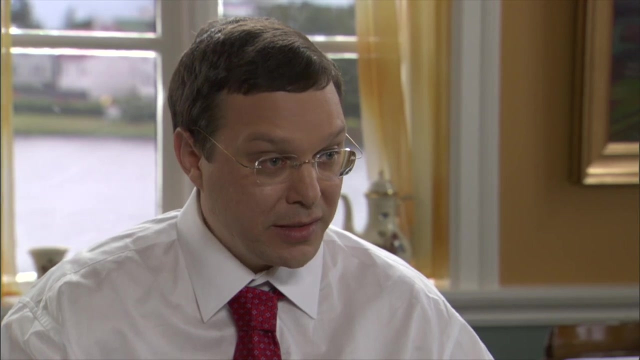 So there were holes, generated artificially by the radiation, in the distribution of hydrogen, And these cavities will appear as dark regions in 21 centimeter maps of the hydrogen, Because the hydrogen was burned out of that region. Exactly right. And so we can not only image the initial conditions of the universe, then the inhomogeneities that existed in it. 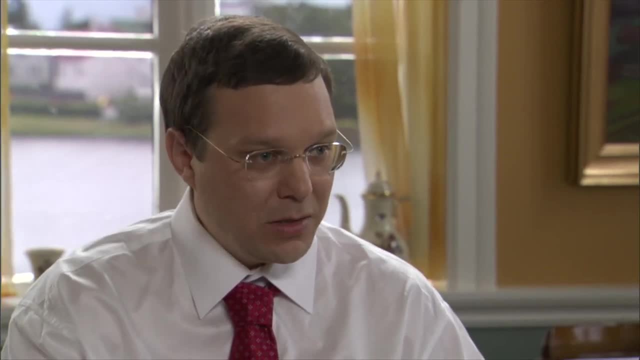 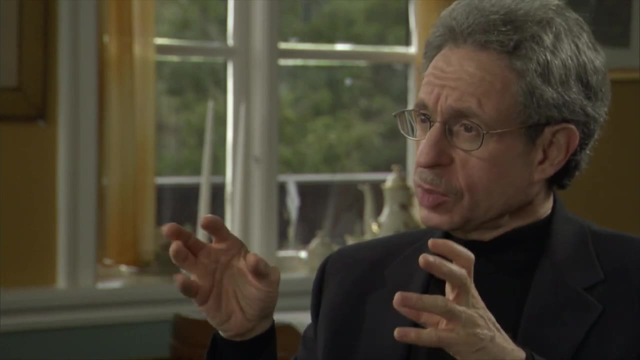 But also the effects of the first galaxies to have formed Inside this gas. Now, will there be any way to do this on a chronological basis, or will you just have one single snapshot? No, in fact Depends where you aim it or focus it. 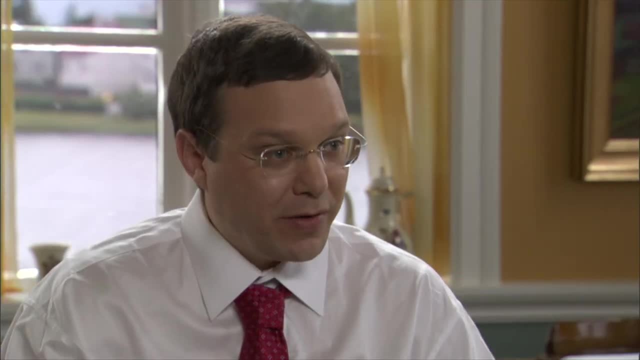 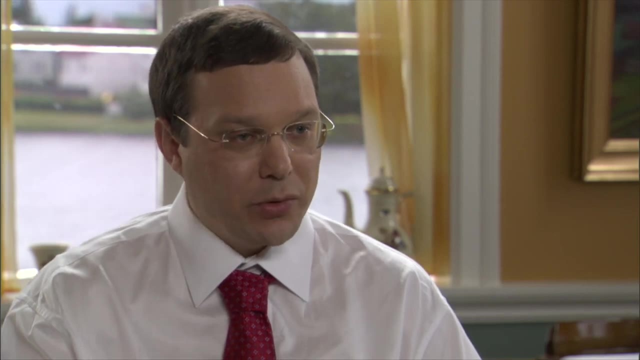 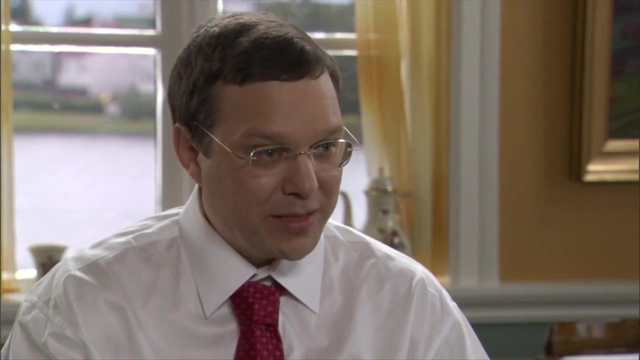 We are looking at the 21 centimeter transition of hydrogen And this wavelength of 21 centimeter is being stretched by the cosmic expansion. So if you are looking at an earlier cosmic time, it's being stretched by a bigger factor than if you are looking at a later cosmic time. 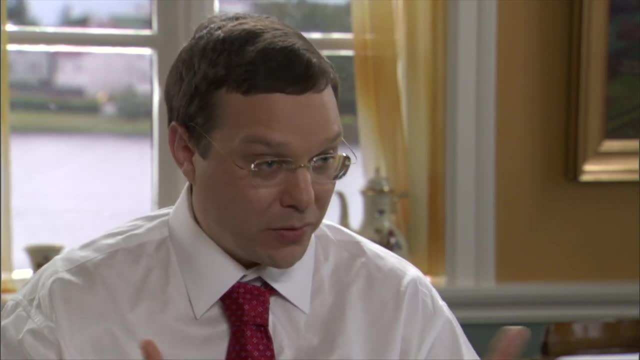 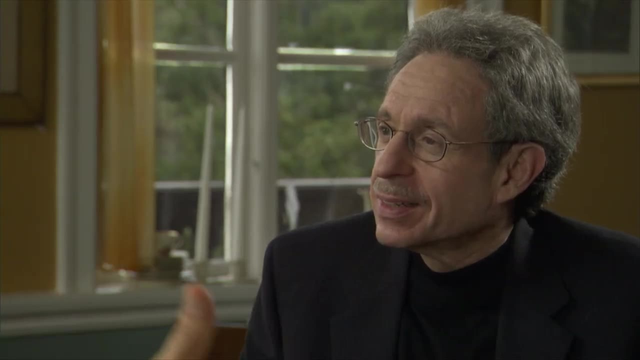 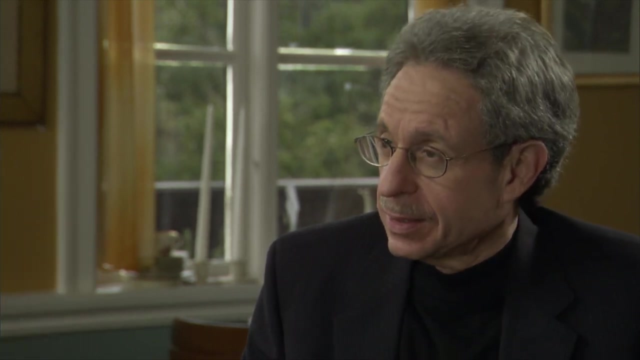 So by observing different wavelengths of radiation or different frequencies of radiation, we are able to slice the universe at different redshifts or different cosmic times, And that's just like slicing Swiss cheese that has holes in it. You will be able to see that the patterns that you observe change. 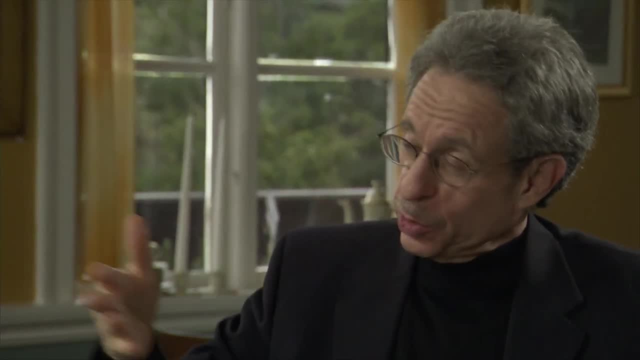 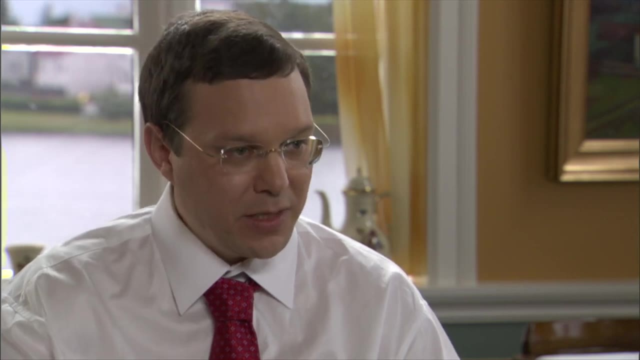 Or a CAT scan of a person which is spatially. you are doing this type of cut temporally over time. Exactly right, So it's three dimensional. We are mapping hydrogen in three dimensions, Both across the sky and as a function of distance from us. 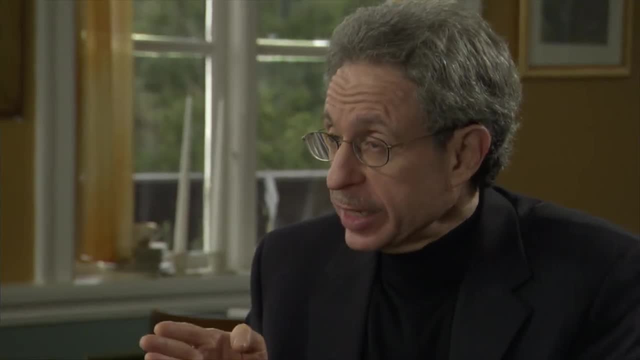 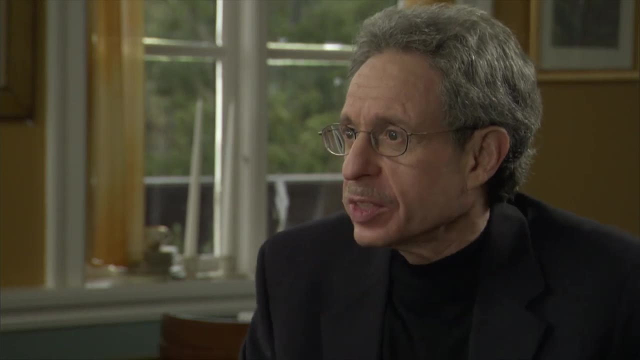 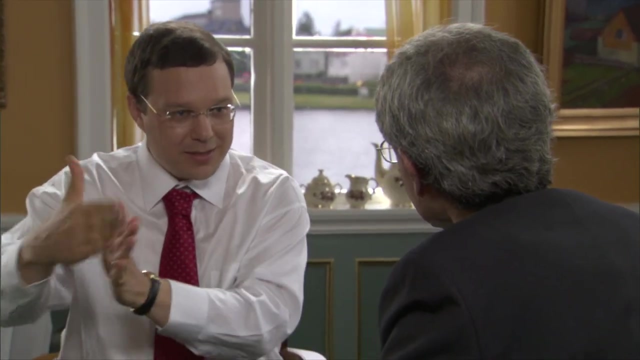 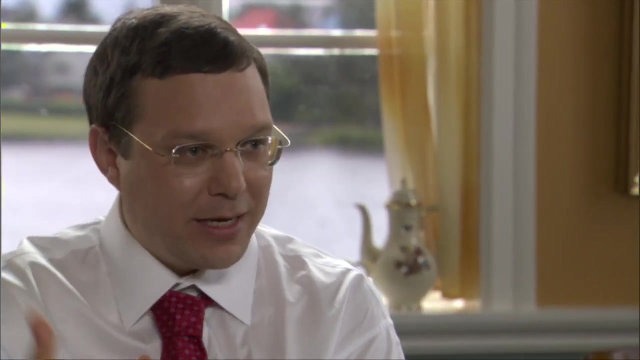 So how accurate can you be in your slicing in terms of depth, which means in terms of time? How fine can we draw this picture? We can, in fact, slice this Swiss cheese of hydrogen in very fine slices, But in order for us to see significant variations, we are adding up slices. 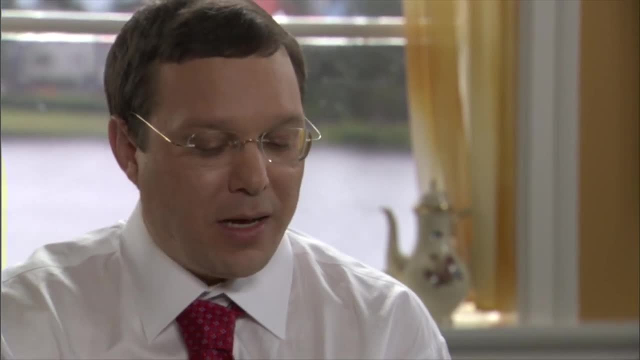 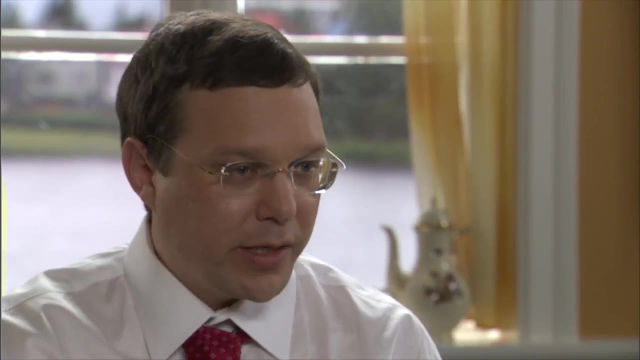 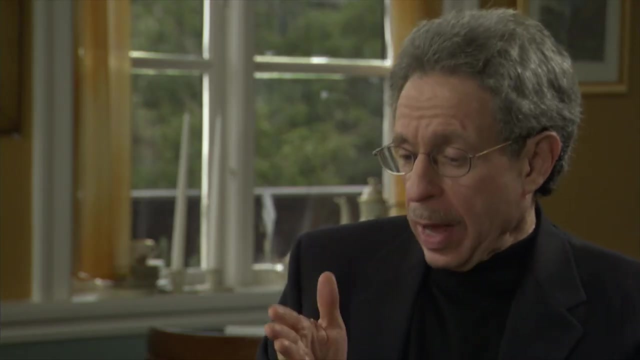 So that we can improve our signal. But we are tuning our resolution on the sky so that it will correspond to the characteristic size of a cavity that was produced by an early group of galaxies. So how much time would then be between images that are reasonably well structured? 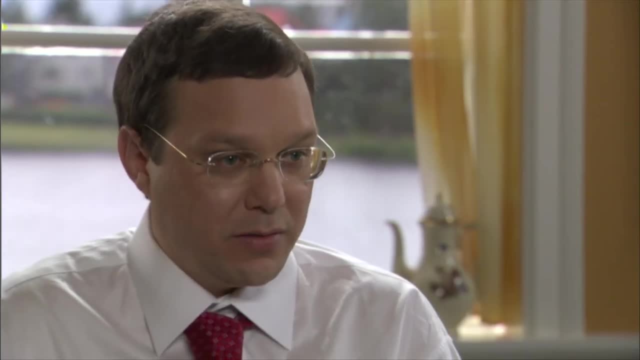 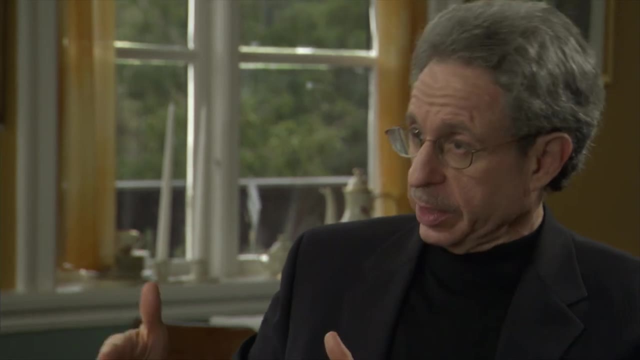 We are talking about tens of millions of years. That's very fine, Very fine Tens of millions If you are looking between, basically, 100 million years and a billion years, into this very interesting period of the formation of first stars and first galaxies. 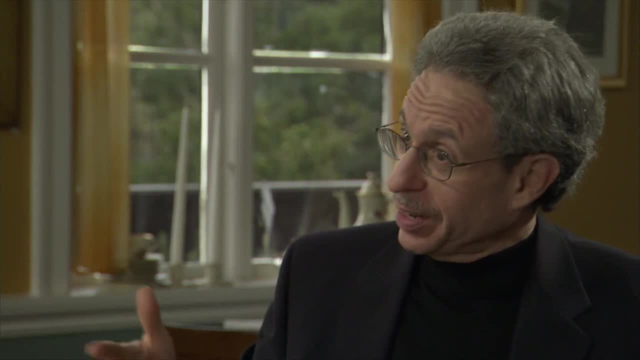 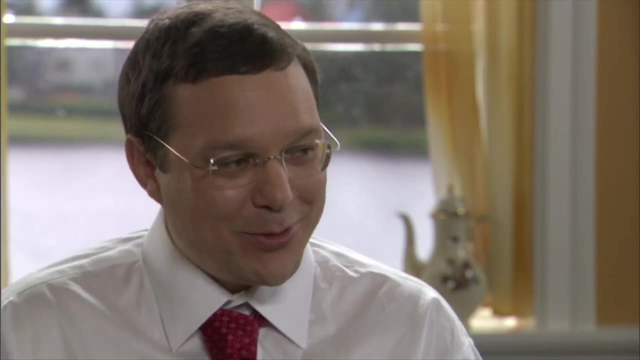 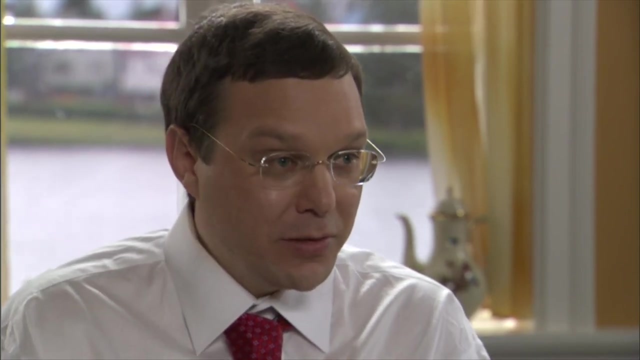 if you can cut that into tens of millions of years, that's really a very fine picture. We are getting a movie of how cosmic structure evolved with time. Now the interesting thing about it: at some point we noticed that the biggest problem is the interference from radio and TV broadcasts on Earth. 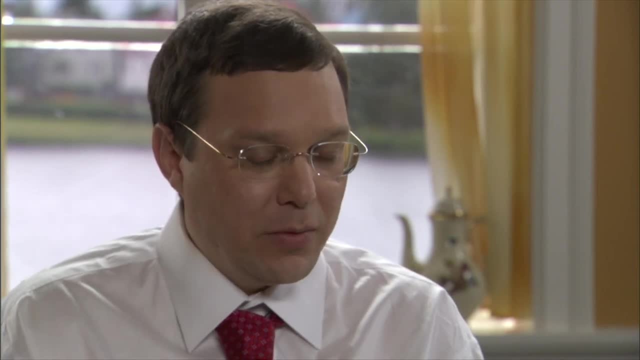 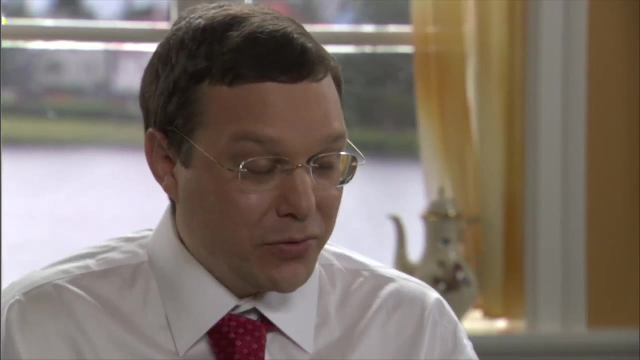 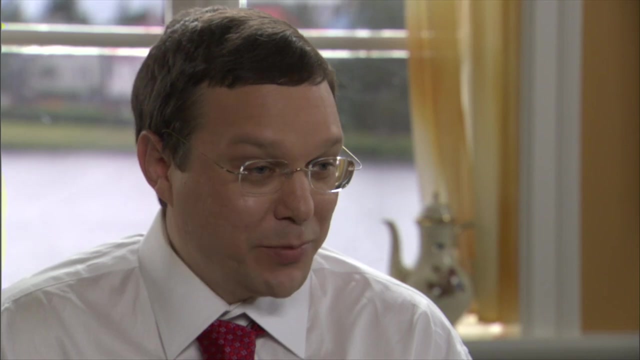 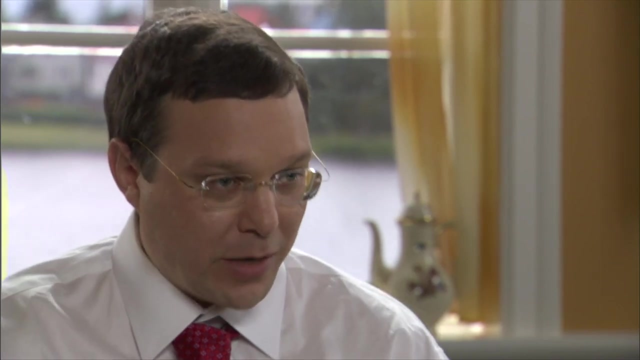 And that's one reason why several of these experiments are being located in remote sites. But then I commented to a colleague of mine that if our civilization is causing us trouble, perhaps we can also put limits on the existence of external civilizations, Because the same data set that we will collect will include information about interference. 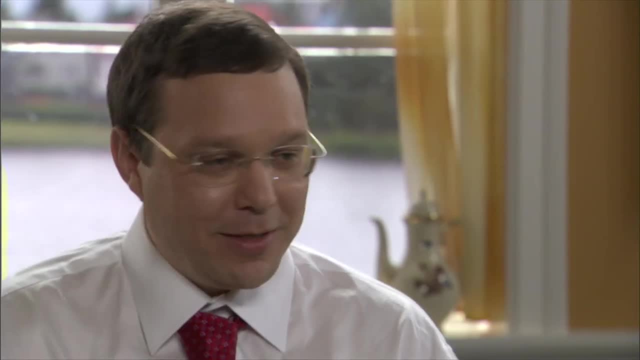 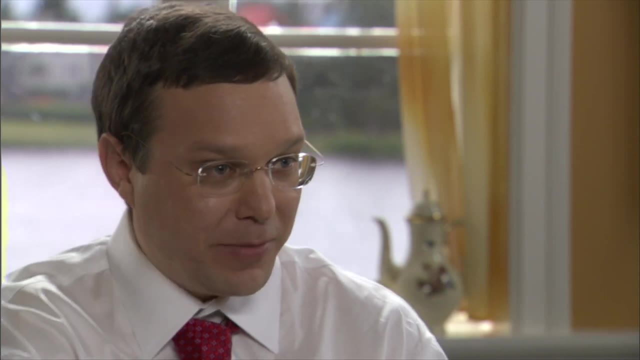 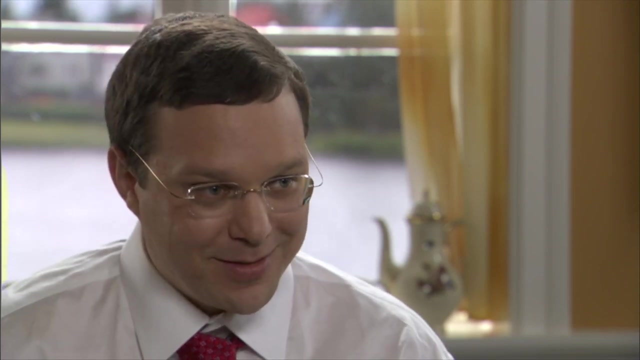 And we did a simple calculation: How far away would you be able to see the Earth as you take such an observatory and place it at a distance? Yes, It turns out that it can be tens of light years. Yes, We've been broadcasting TV and TV shows, radio shows and as well as we've been using military radars for over 50 years. 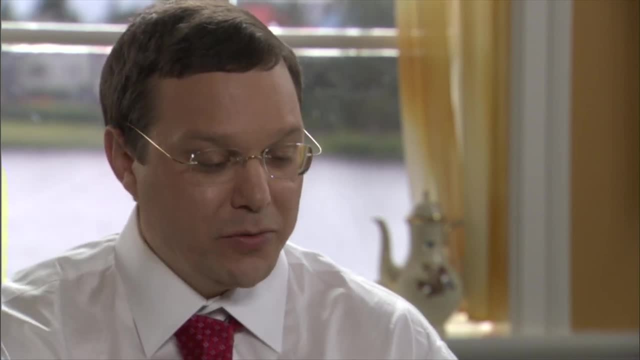 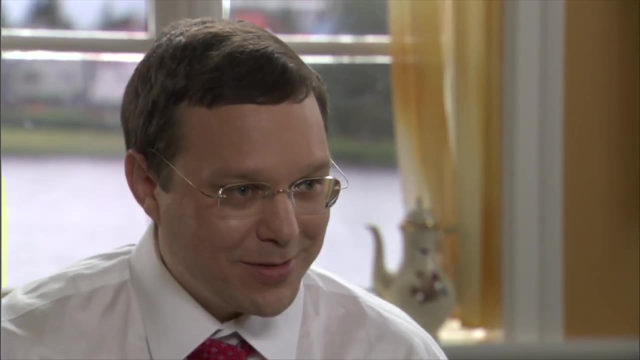 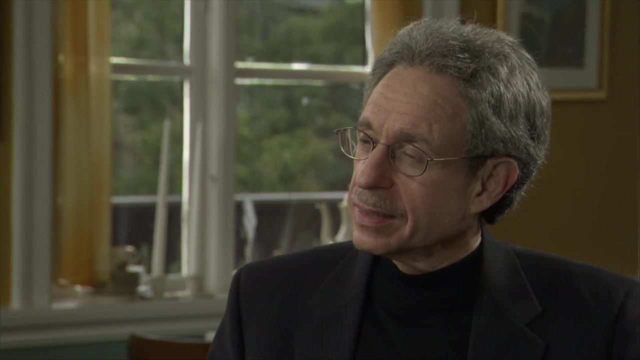 So that means that the signals that we receive, the signals that we receive, the signals that we receive from the Earth, it turns out that the signals that we produced were able to reach distances of 50 light years, And with the kind of observatories that we are now constructing, you could see the Earth from those distances. 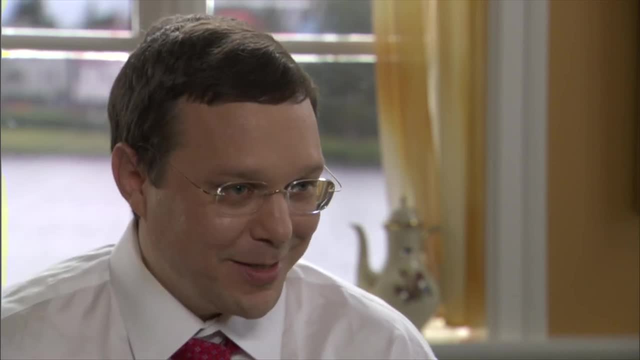 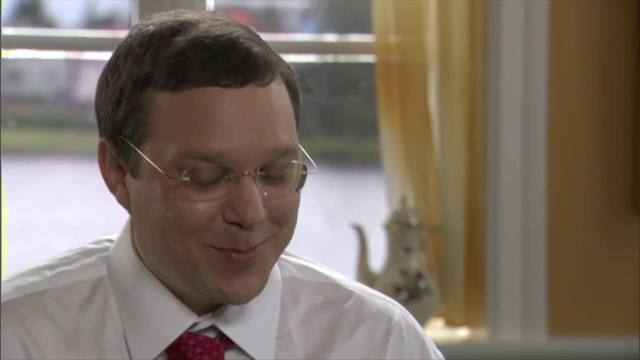 So if there is anything out there, they may pick up the signals and be able to tell that we exist. I hope they're nice, Me too, But based on our own experience, the strongest signals that we produced were from warning systems for ballistic missiles. 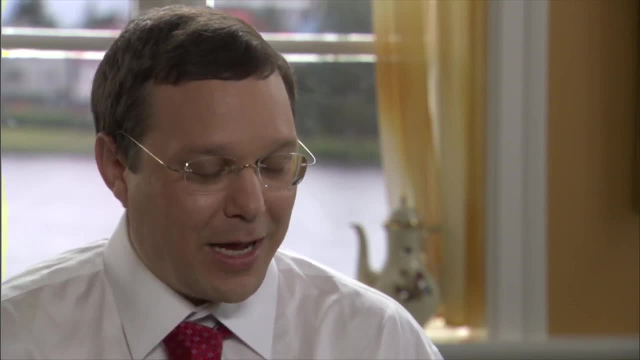 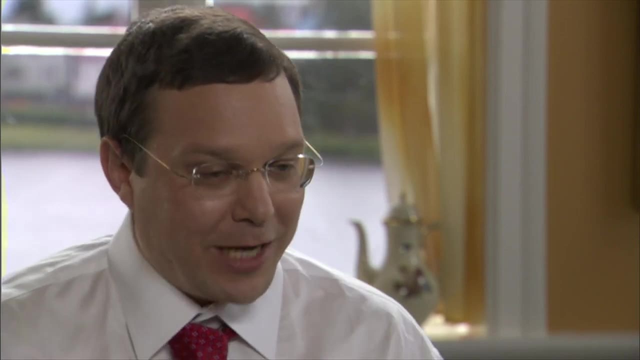 And if I had to guess, I would say that the brightest civilizations that may exist- of course, we don't know if anything exists out there, but the brightest ones are probably militants-